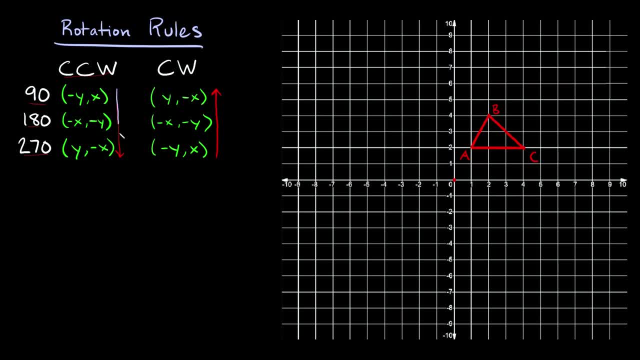 comma negative x. Okay. so again, if you can memorize one set, it'll be the same thing going down as it is going up. Okay, now, how do you actually go about rotating and using these rules right here? Okay, well, the first thing you have to do is just write down the coordinates of each of the points on 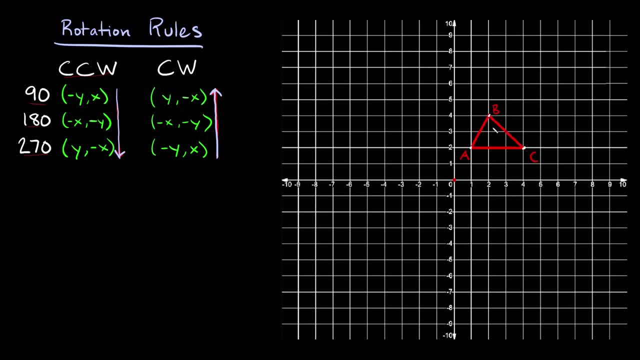 whatever shape you're trying to rotate. So here we have a triangle. right, so we have three points: a, b and c. Okay, so we're going to write down the coordinates for these three, right here. Okay, so a right here is at 1 comma 2. right, so a is at 1 comma 2, b is at 2 comma 4, 2 comma 4 and then c. 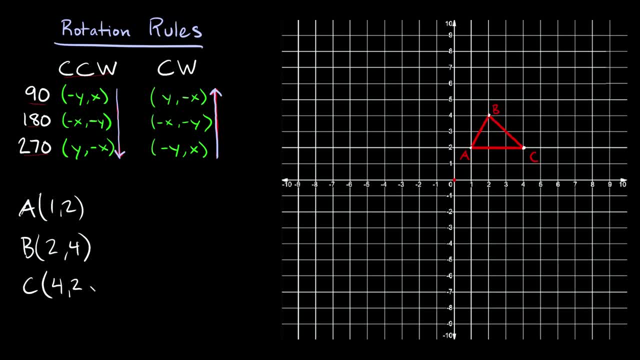 is at 4 comma 2. all right, Okay. now let's say we were asked to rotate this triangle 90 degrees in the counterclockwise direction. Okay, well, I'm going to come over to my little rules over here, So I'm going to rotate in. 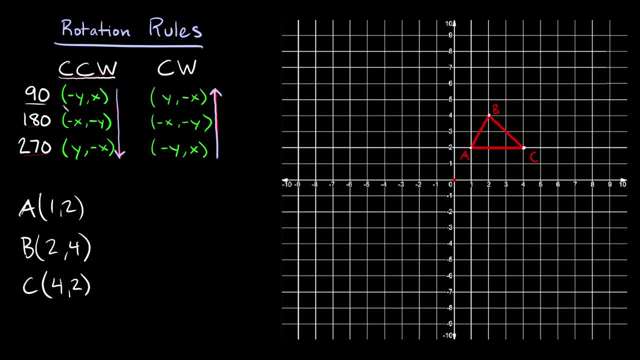 the counterclockwise direction, 90 degrees. right. so that means I'm going to use this little rule right here: negative y comma x. Okay, so first of all, these points right here that we just wrote down, they are in the form x comma y, right. but now, since we 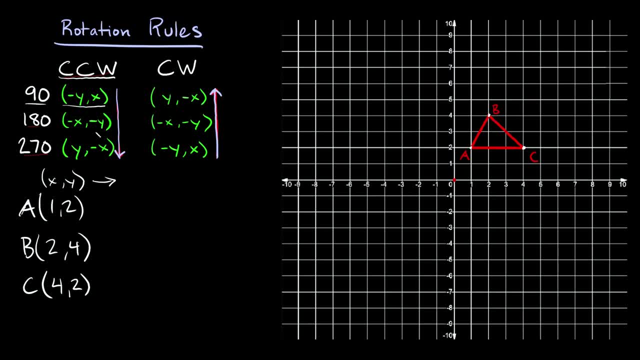 are going to rotate them. we're going to rotate them into again this rule right here: negative y comma x. Okay, so let's rotate this first point right here: a. so it's at 1 comma 2.. Okay, but when we rotate it or transform it, it's going to be at as you can see, we are going to write the y. 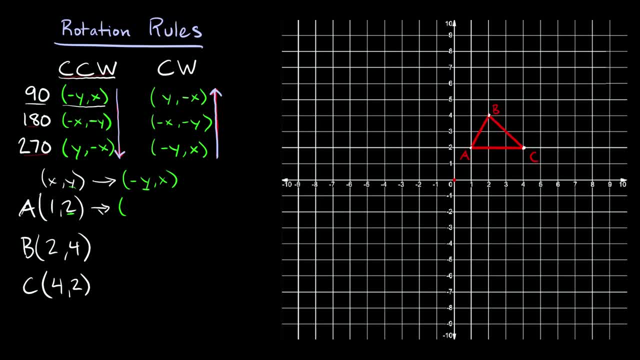 coordinate first, right. so our y coordinate here is 2. so we're going to put a 2 here first and we're also going to change the sign, Okay. so over here it's positive, so over here it's going to be negative, All right. and then we're going to write our x coordinate last. so our x coordinate here is: 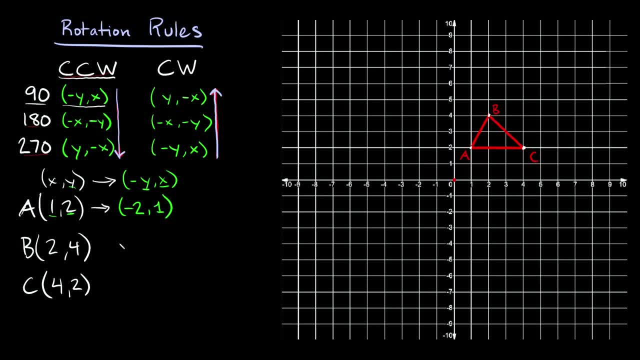 a 1, so we're going to put a 1 right there, Okay. so then let's do the same thing with b. So again, we're going to write our y coordinate first and we're going to flip the sign. so here, this is a positive. 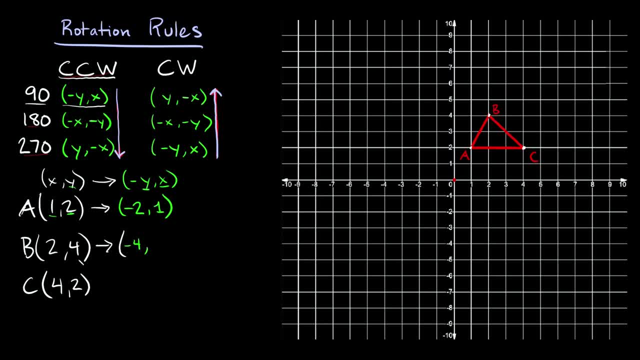 4. so then here we're going to have negative 4 and then we're going to have a 2. at the end, right, our x coordinate, And then lastly c. right, here again, write the y coordinate first, so that's a 2.. 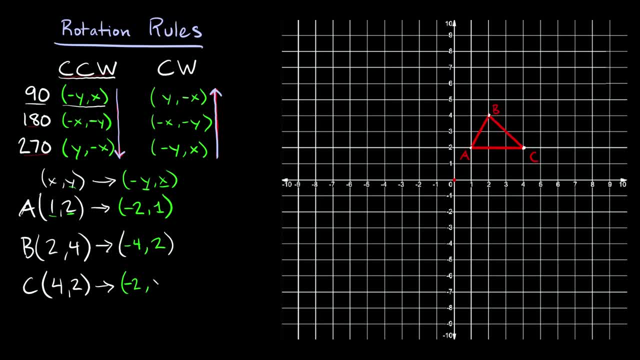 And then flip the sign, so negative 2, and then here we have our x coordinate of 4.. Okay, so then here's our three coordinates. so this coordinate right here is basically a prime, this coordinate right here is b prime and this one is c prime. Okay, so then we just have to graph these three. 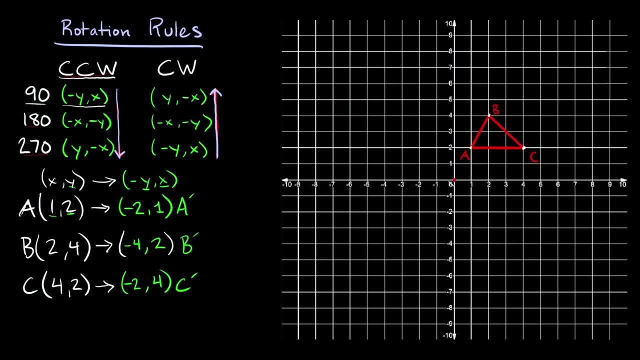 points now. All right, so then again: a prime is at negative 2, 1, right, so negative 2, 1 is right there. b prime is at negative 4, 2, so negative 4, 2. and c prime is at negative 2, 4, right, negative 2, 4.. 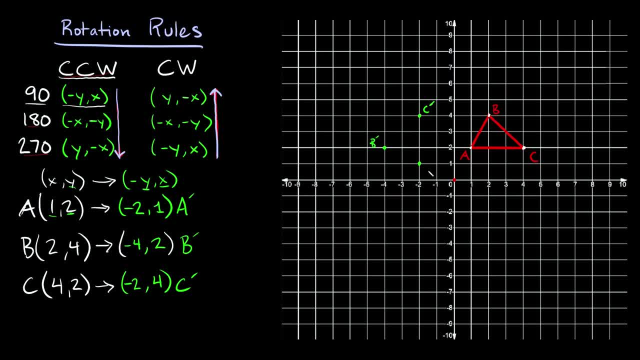 So again, that's c prime, this is b prime and this is a prime. Okay, and then we just have to play, connect the dots right. So here is your triangle, rotated in the counterclockwise direction 90 degrees. All right, so hopefully that wasn't too bad. let's try another one. So here we have triangle. 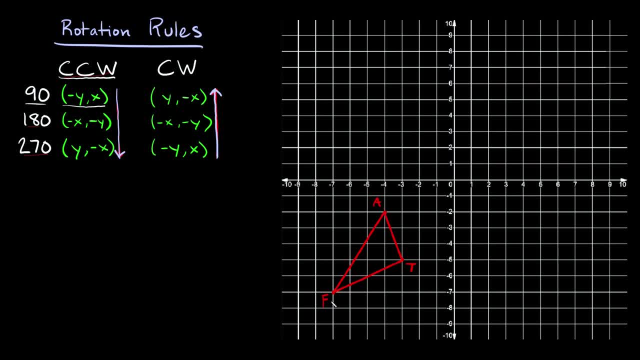 FAT, all right. and this time, let's say, we were asked to rotate it 180 degrees in the clockwise direction. Okay, so clockwise direction, 180 degrees. and remember, 180 degrees is the same exact thing for counterclockwise and clockwise, so it doesn't actually matter which one we use. But again, keep in mind, this is our starting position. 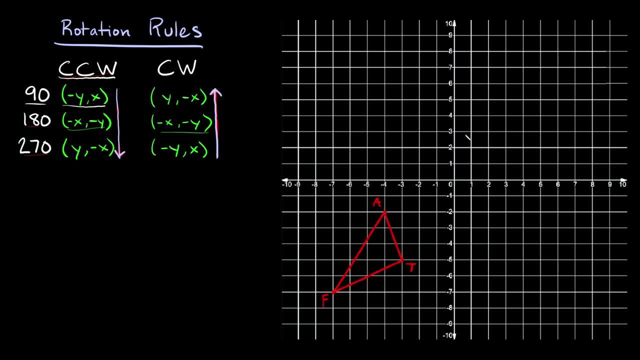 so a 180 degree rotation should wind us up over here, right on the opposite end. So the first thing you want to do is just write down your coordinates for each of these, right? so for F, A and T: Okay, so, first of all, F is at negative 7. 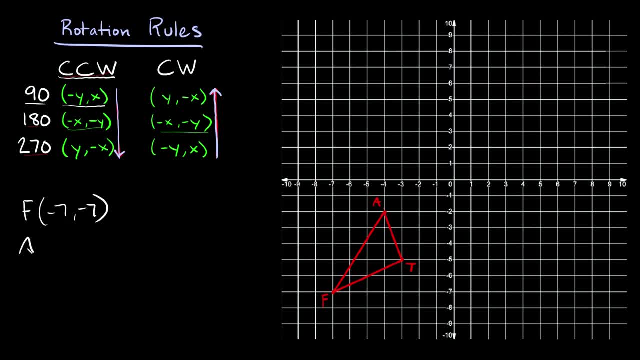 negative 7, all right, negative, 7, negative 7. A is at negative, 4, negative, 2, negative, 4, negative, 2 and T is at negative, 3, negative, 5.. All right, T is at negative, 3, negative, 5.. Okay, and the rotation. 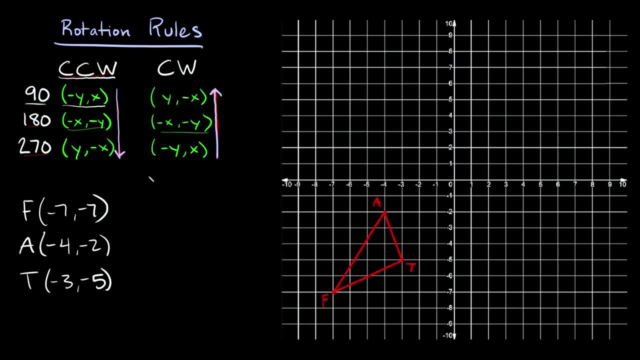 rule that we're going to use is this one: right here, right, so negative x, negative y. So remember, we're starting as x comma, y, right, that's how we always start, and then, in this case, we're going to transform it to that right: negative x, negative y. Okay, so this is going to be. 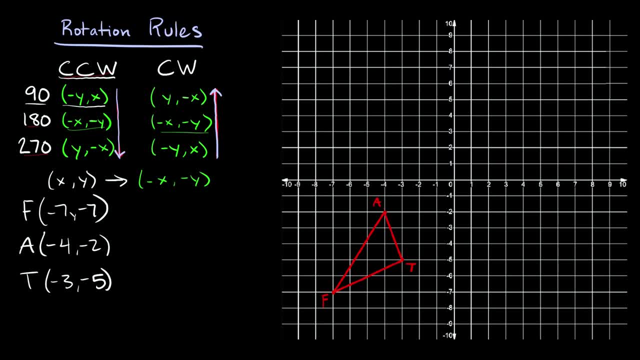 easy. all we have to do is change the signs on each of our x and y's, right, It's still going to stay as x, y, like normal, but we're just going to change the signs on all of them, Okay. so then, for example here we have: F is at negative 7, negative 7. so then F prime is going to be at positive 7. 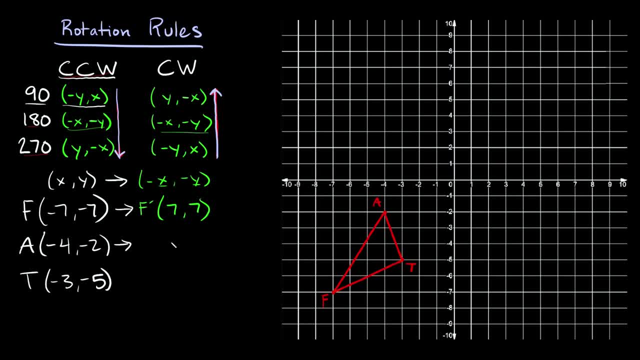 positive 7. right Now, A is at negative 4, negative 2, so A prime is going to be at positive 4, positive 2.. Okay, and then, lastly, we have T right here at negative 3, negative 5.. So then T prime is going. 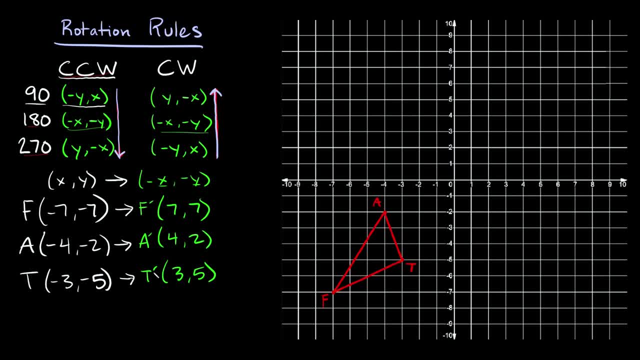 to be at positive 3, positive 5.. All right, so then we just have to graph these really quick. So F prime is at 7, 7 right, so 7, 7.. A is at 4: 2, so 4, 2.. 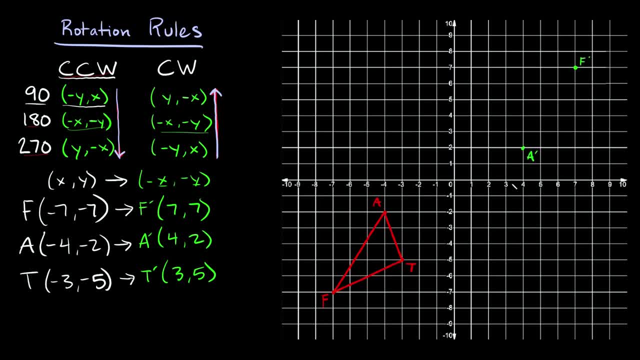 That's A prime, right, that's F prime. and then T is at 3, 5, so 3 comma 5.. All right, so that's T prime. Then the last thing you have to do is connect the dots. Boom, boom, boom, All right. so here is your. 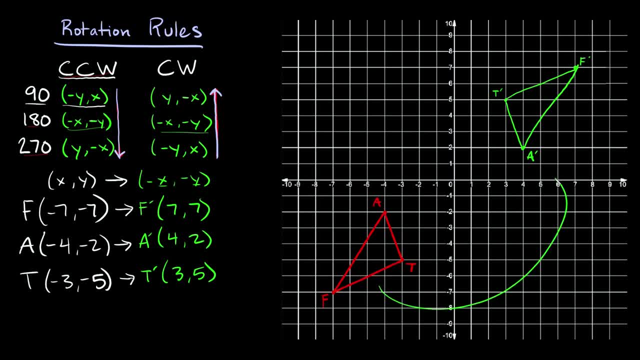 triangle rotated in the clockwise direction. Boom, 180 degrees. Okay, so here's the last example. So we have this quadrilateral and let's say we were asked to rotate this 270 degrees in the counter clockwise direction. All right, well, first of all, you can see that this shape, right here it crosses. 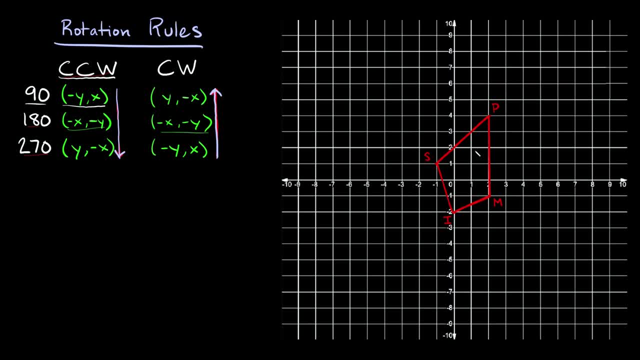 the x-axis and the y-axis. So you can see that this shape right here, it crosses the x-axis and the y-axis. So you can see that this shape right here, it crosses the x-axis and the y-axis, All right. so you can see that this shape right here, it crosses the x-axis, All right. so it's not in its own like. 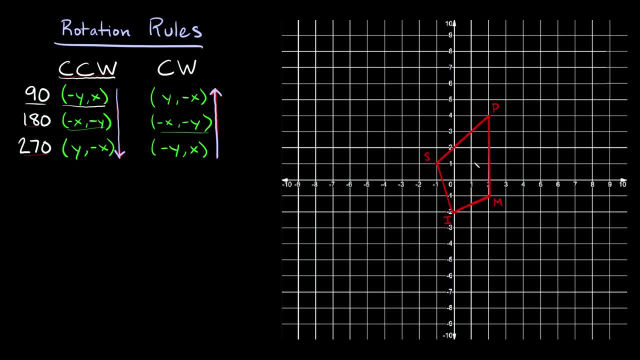 little quadrant anymore, So it's going to be a little more difficult to tell if we rotated it correctly, but we're still going to just use our rotation rule. All right, so our rotation rule for 270 degrees in the counterclockwise direction: is this one right here? So y comma, negative, x, All. 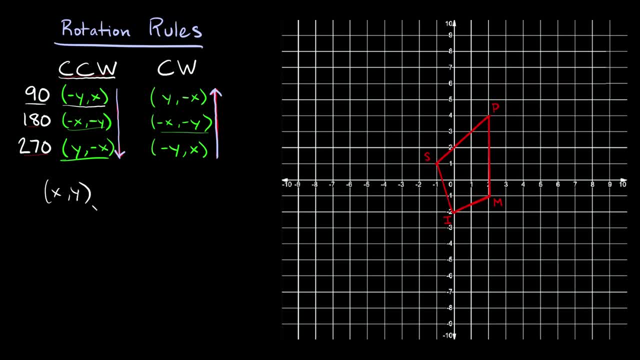 right. so again, we always start as x comma y right, and then we're going to transform it to y comma, y comma negative x. Okay, so let's write down our points. So first of all, s right here. s is at negative 1 comma 1.. i is at 0 comma negative 2.. All right, 0 comma, negative, 2.. Let's see: m is at 2. 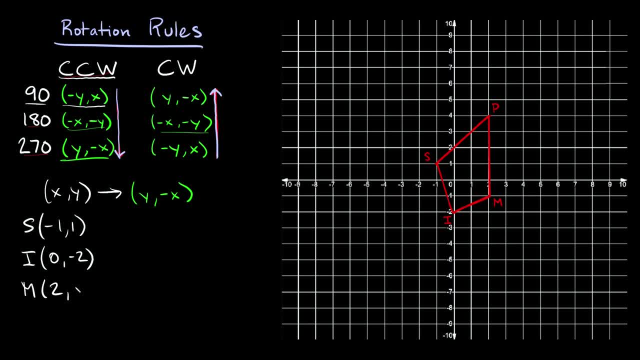 comma negative 1.. m is at 2 comma negative 1.. And then, lastly, p over here is at 2 comma 4.. Okay, 2 comma 4.. All right, so then we're going to switch this one. So here we're going to write the y. 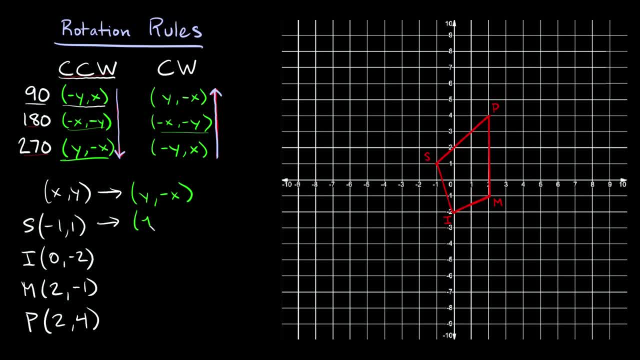 coordinate first, right. So the y coordinate here is 1.. So it just stays as 1.. And then we're going to write our x coordinate and flip the sign. Okay, so here we have a negative 1.. So over here it's. 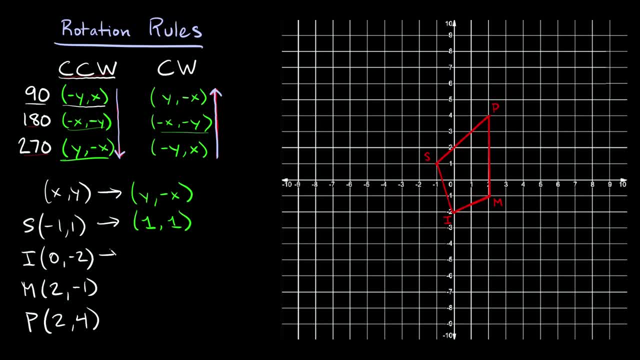 going to turn into positive 1.. Okay, now here same thing. we're going to write our y coordinate first, which is a. let's change it to green, negative 2.. And then our x coordinate. change the sign a bit. We just have a 0 here, so it's just going to stay. 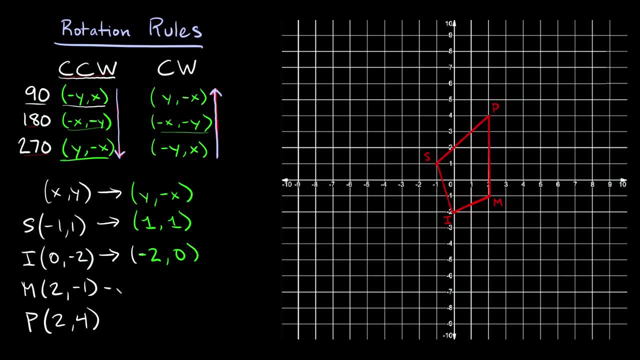 0. There's no sign on 0. And then m right here. So again write the y coordinate first, So negative 1, right negative 1.. And then change the sign on your x coordinate So it's going to be a negative 2. 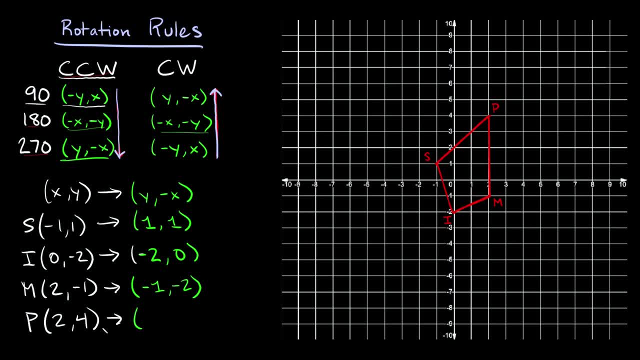 over here. And then, lastly, p. right here, Our y coordinate is 4 and our x coordinate is a 2. So we're going to flip the sign, So it's going to be negative 2.. Okay, so, here we have s prime, Here we have i prime, Then m prime and p prime. Okay, so let's. 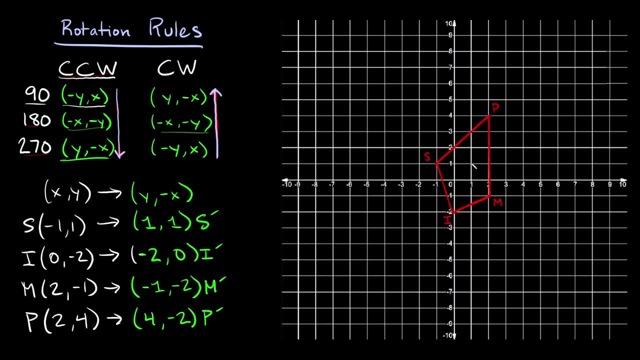 graph these right here. So s prime is at 1 comma 1.. I prime is at negative, 2 comma 0.. Negative, 2 comma 0.. And let's label these s prime. i prime And then m prime is at negative 1, negative, 2.. 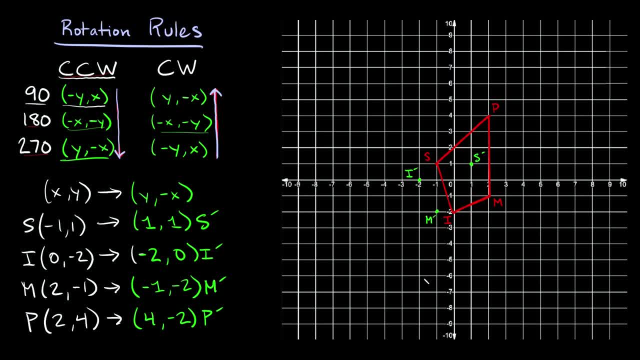 Negative, 1 negative, 2. That's m prime, And then p Prime is at 4- negative, 2.. Right, 4 negative, 2.. All right, and then again, the last thing you do is just connect the dots. All right there? Okay, so we. 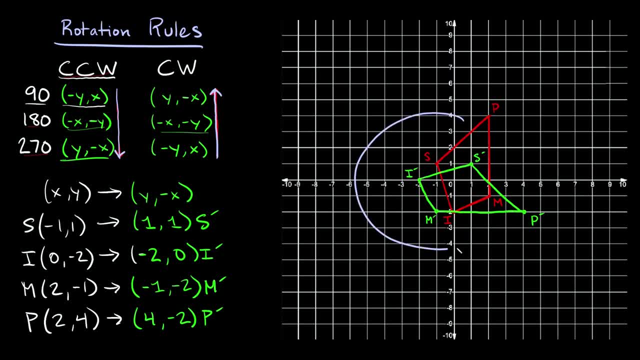 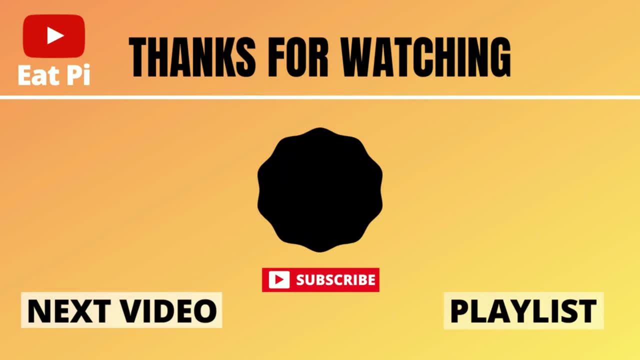 just rotated this shape 270 degrees in the counterclockwise direction. So if you found the video helpful, definitely leave a thumbs up down below, And if you have any other questions or want to see any other examples, just let me know in the comment section. below.